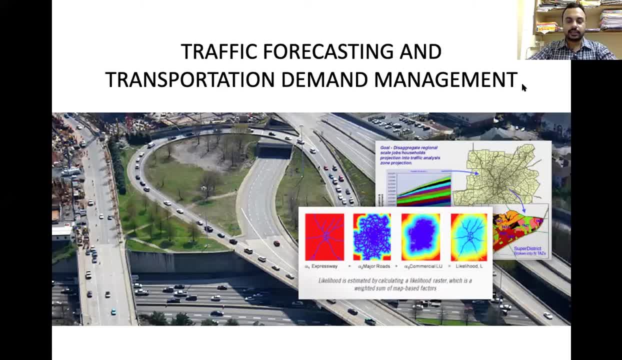 So population forecasting- It is also an important part of traffic forecasting. Now, what are the other factors that play a great role in traffic forecasting? It may be the generation of population, It may be urbanization, It may be amount of job creation. 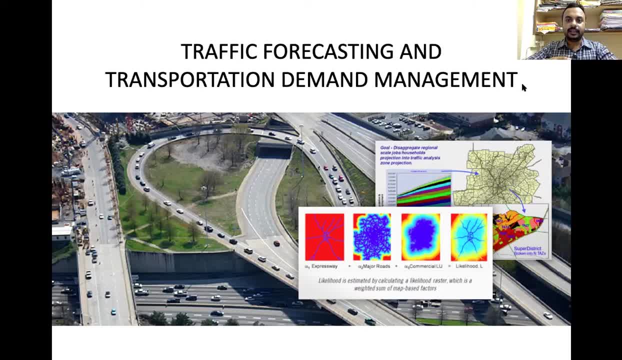 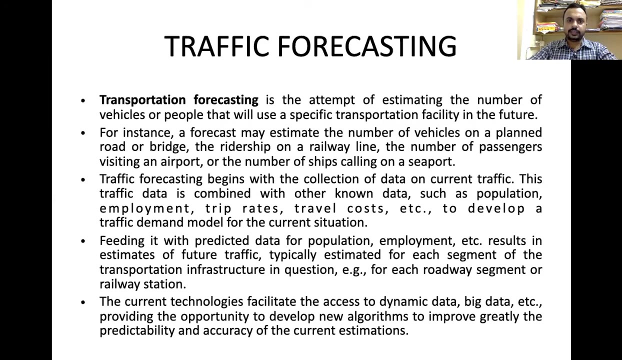 It may be the other facilities, Like if we observe that there is a development of metro, rail or other such kind of facilities being developed, then that affects the traffic in the future time. Okay, So let us see So. as we all know that traffic forecasting, it's an attempt to estimate the number of vehicles. 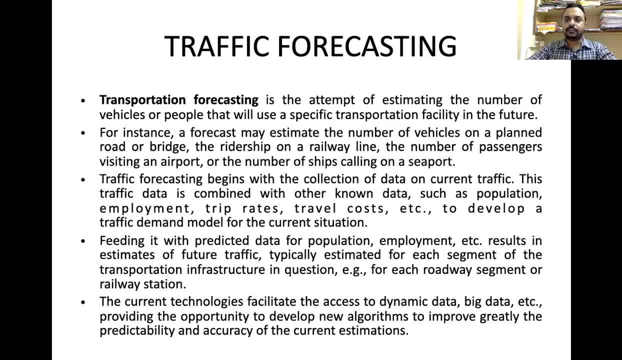 or people that will use a specific transportation facility in the future. Traffic forecasting plays a very, very important role in the analysis of transportation planning. Okay, So a forecast may estimate the number of vehicles, the number of vehicles on a planned road or a bridge. 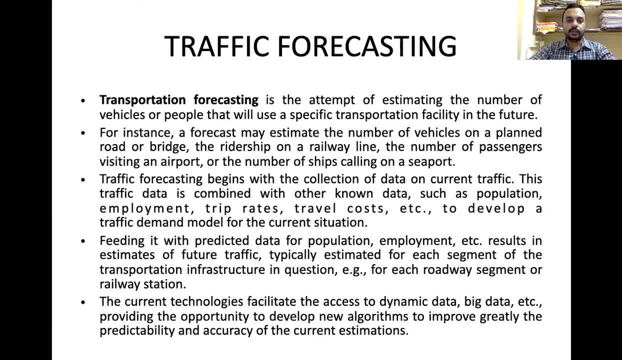 the ridership on a railway line, the number of passengers visiting an airport or the number of ships calling on a seaport. See, all these things are interrelated. If the number of passengers are increasing on the railways, if suppose the number of passengers reaching Guwahati is increasing in the railways. 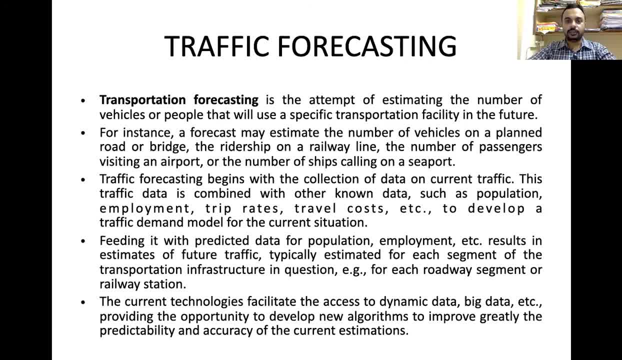 that will affect the transportation number of people using the road, Isn't it? If the number of people using the airport has a drastic increase in the number of people using the airport, that will also affect the number of people using the roads. Okay, 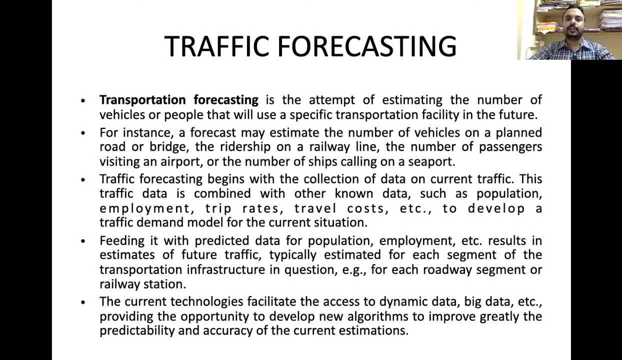 If an increased facility in the airport leads to an increased number of air travelers and which also leads to an increased number of taxis flying to the airports, Okay, All these things are interrelated. The traffic forecasting: How do we do the traffic forecasting? 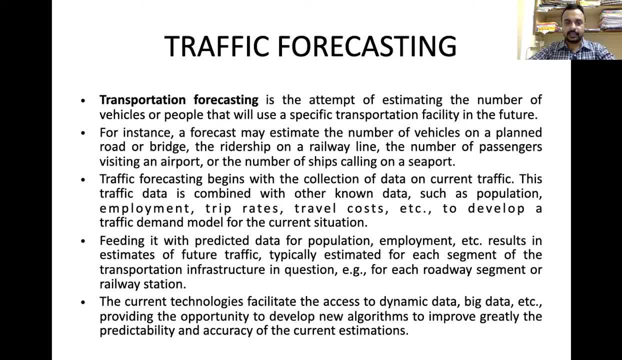 Before doing the forecasting, you should have the existing data. The process of forecasting begins with the collection of the data on the current traffic. This traffic data is combined with other known data such as population, employment, trip rates, travel costs, etc. 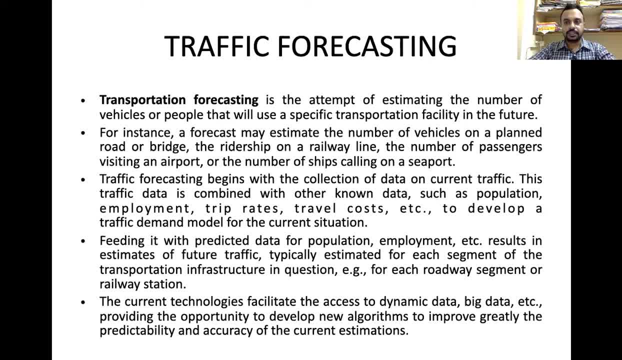 to develop a traffic demand model for the current situation. Okay, The, what are the? what is the cost of traveling? What is the rate of employment generation? All these plays a very, very important role in the forecasting of traffic And when we have all this data, feeding it with predicted data for population, employment, etc. 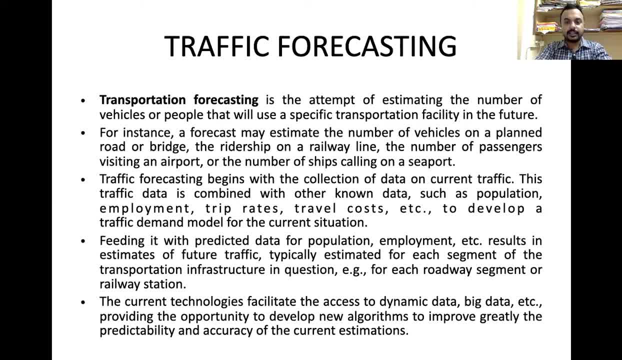 results in the estimates of future traffic, Typically estimated for each segment of the transportation infrastructure in question. Okay, So We have software, We have resources where we can now analyze the dynamic data. We can analyze the big data Once we have all the data of population, transportation costs, employment, present traffic. 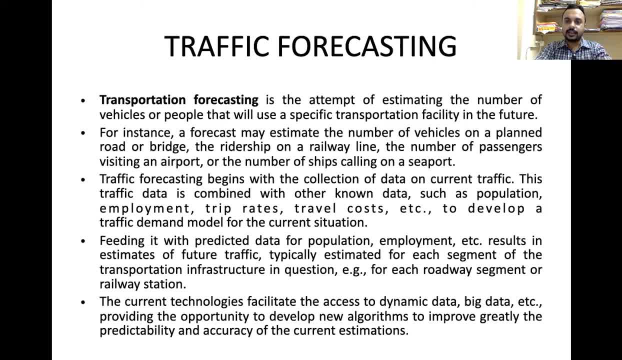 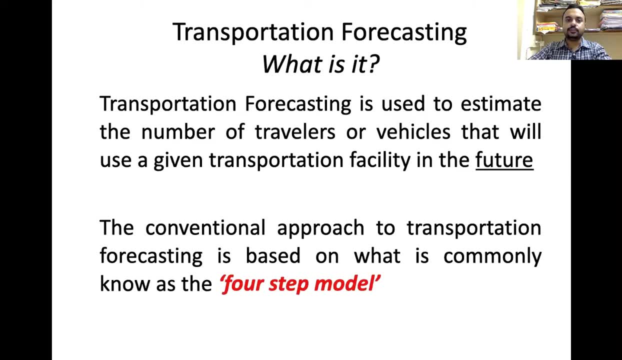 we can model it to forecast the traffic to be occurring in a future date. Okay, And then we can do the transportation planning. So Why is transportation forecasting done? It is used to estimate the number of travelers or number of vehicles that will use a given 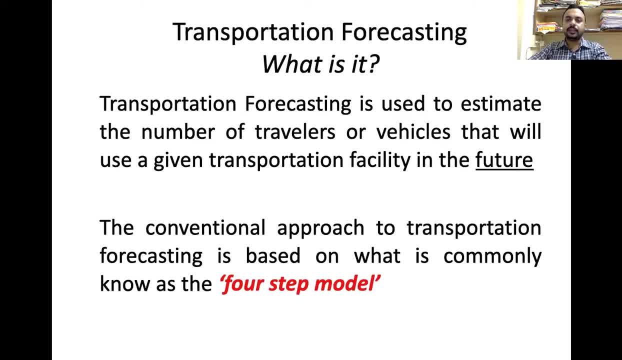 transportation facility in the future. Okay, So, as I have already said that the transportation planning process is a four-step model, We'll study in detail about this four-step process. So I hope it is clear that transportation forecasting plays a very important role in 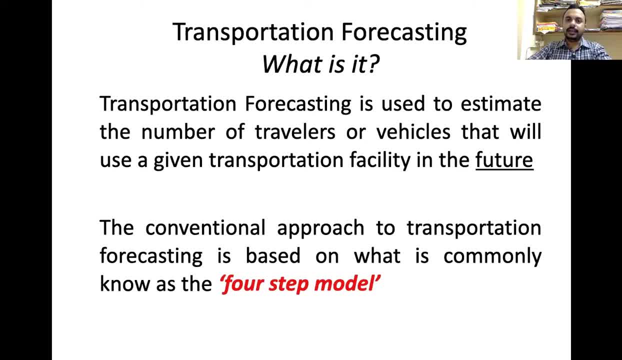 the construction of transportation facilities. Now, for example, an engineer or transportation planner says that in this particular route we need a flyover. Okay, So, my dear friends, one flyover. may the construction cost of a flyover, maybe some 400 crores, to 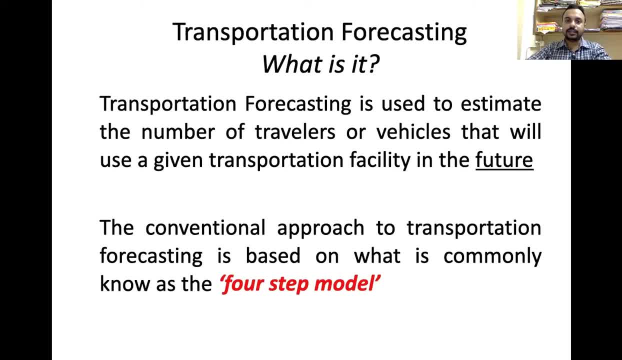 1000 crores, depending upon the place where it is constructed, depending upon its length. Okay, So, Before investing such a huge amount of money, as a planner or as an engineer, You must, You must be able to know whether this type of facility will sustain in the future. 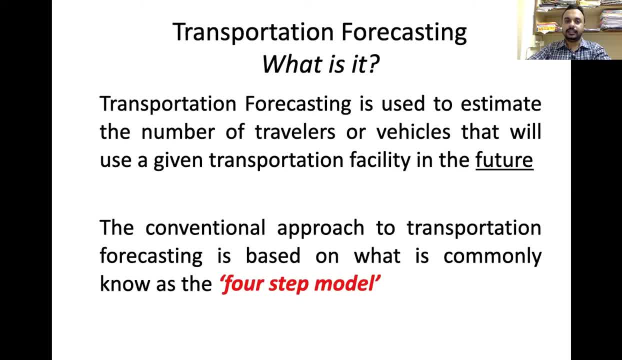 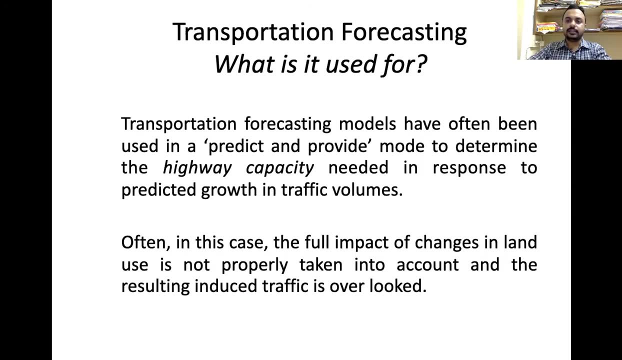 You cannot construct another flyover after two or three years. So before using or before constructing that facility, we should be able to predict about the future. And that is nothing but the transportation forecasting. So transportation forecasting models have often been used in a predict and provide mode. 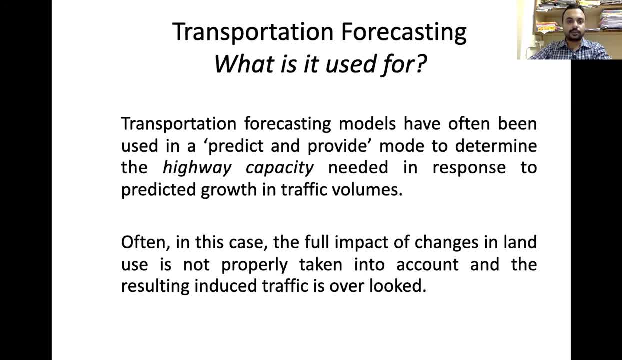 to determine the highway capacity. And so, when we talk about transportation forecasting and transportation forecasting, the first step for transportation forecasting is to regulate the traffic speed And the second step is to decide what type of traffic speed we are not actually going to use for our transportation. 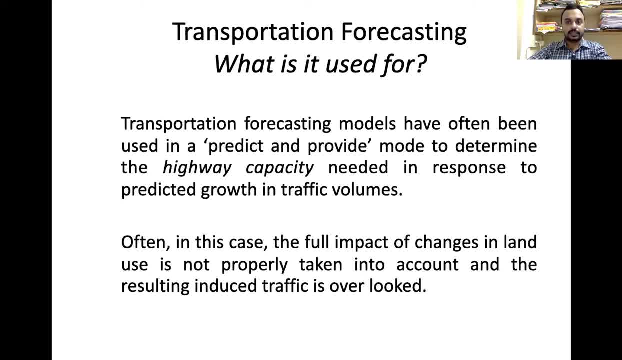 What type of traffic speed we should be able to use, What kind of traffic speed used by our transportation. We have already studied these two types of traffic speed, Like traveler speed, traffic density and speed. What traffic speed? What are all these? 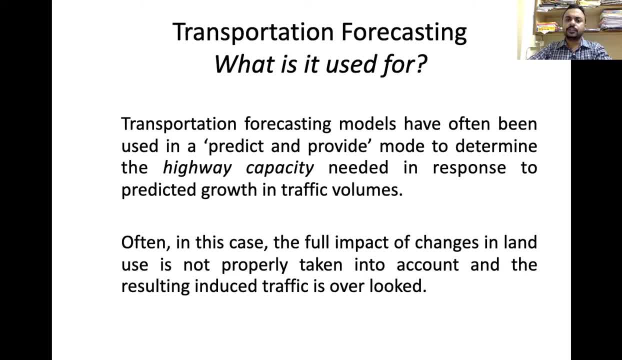 These are the macroscopic parameters. Very, very important macroscopic parameter: What type of speed we generally use? Time mean or space mean. we have already studied about highway capacity also in our previous lectures. so to predict the highway capacity in the future we can use the method of traffic forecasting. okay, there is. 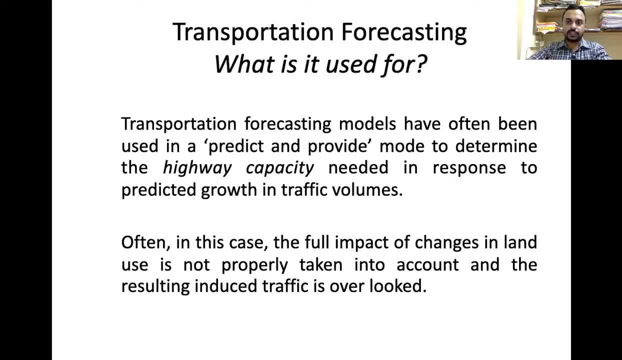 another thing that what is the impact of this? transportation facilities in the land use pattern? okay, a land area is used for various purposes. it may be used for the construction of roads, for development of shopping complexes, for development of some other business areas. so when you construct a facility in a road that affects the entire area. if you have better roads, there will be more. 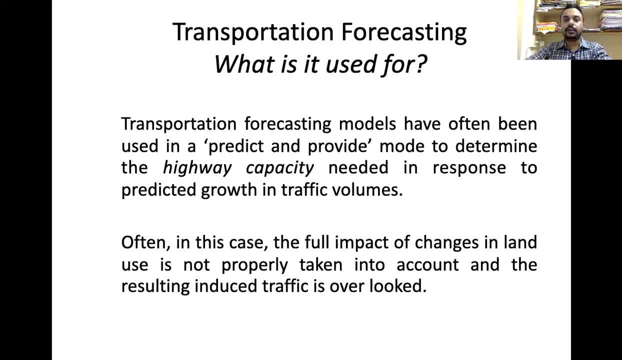 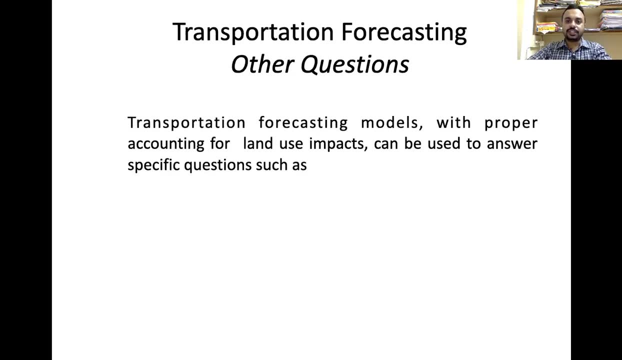 development again. with more development, there will be more traffic, okay, so I hope that it is clear why, how these things are going to be implemented in the future. so thank you very much for your attention. thank you very much for your attention. um, people do not feel to take that particular road. okay, if there is, and with traffic jams and traffic. 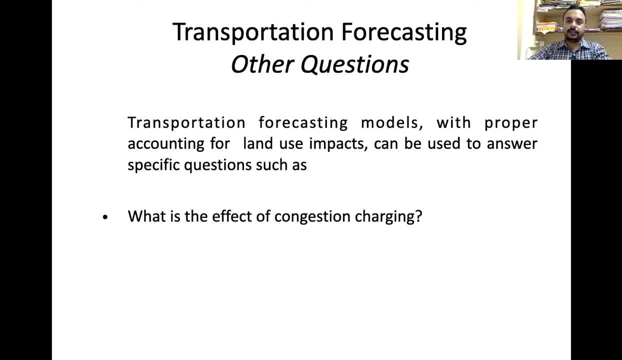 concessions, your amount of money required to travel from one place to another increases. if you have to frequently stop in because of traffic jams, you will have to spend more money in traveling, isn't it? so that is a demotivating factor. what is the effect of parking control and transportation? 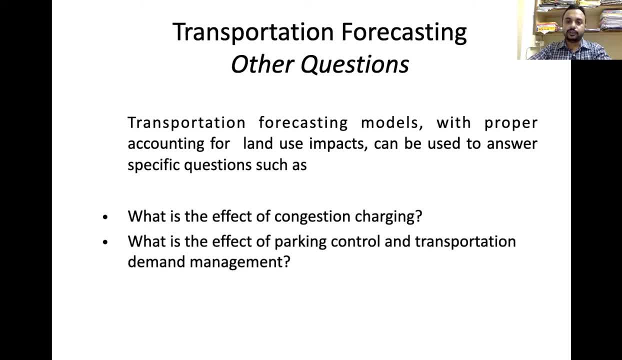 demand management. if, as a planner, you can control the parking, okay, we can see. if you go to a any city, any city, you will see that there are places where there will be unorganized parking. so this unorganized parking hampers the traffic flow. so if you construct some organized parking facilities, that is also that it will also have. 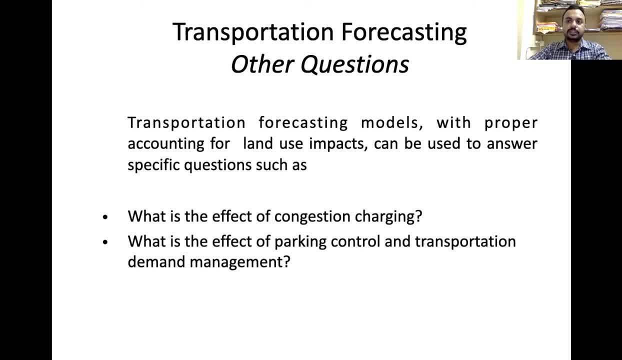 a huge impact in the transportation or in the traffic in the future. okay, what is the effect of more concentrated development? if an area is develop, it developed. so what is its effect? okay, if some huge amount of industries or, what to say, offices are coming in a particular 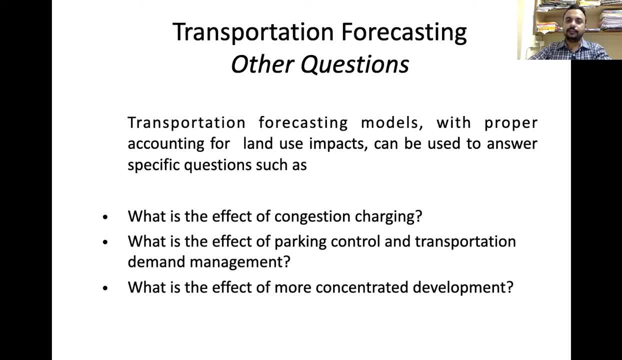 area, then obviously the effect will be there will be huge number of demand of transportation facilities in that particular area. okay, so all these things are interrelated. if there is business, there is a need of for transportation. if there is good transportation facilities, there is an income of good business in that particular area. okay, dear friends, now we will learn about the. 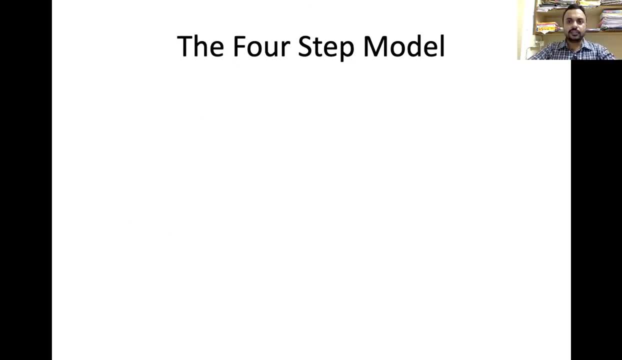 four-step model of transportation planning. see this four-step model I will discuss briefly here. we will discuss step-by-step processes in the latter classes, but you must be able to know about the importance and of each and every step in this four-step model. okay, so the first step is: 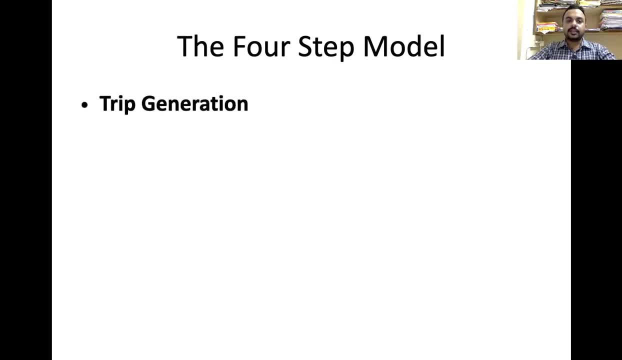 trip generation. okay, so what is trip generation? it is, it estimates the number of trips from given origins and destinations. okay, so what does it mean? that how many numbers of trips are generated from a particular place? okay, suppose there is a place called a, from a, the, how many trips are generated? 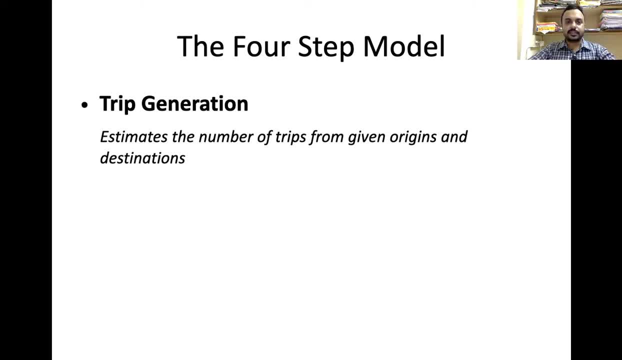 in a particular day, for example from a, there will be five trips generated to location b, five to c, seven to b and likewise okay. so if you divide one particular zone area into several zones, suppose one area is divided into ten zones, so there will be trip inter journal trips also there. 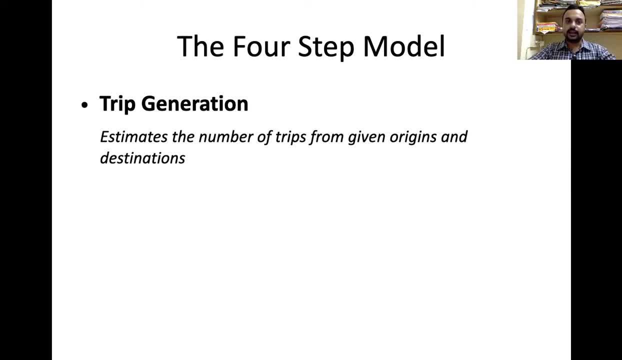 will be trips which will go outside the zone area also. okay, that is trip generations. how many trips are generated from a particular area, from this area? if they're, suppose, 100 trips, that means we do not know where they are going, but 100 trips are generated. now if we study about where these trips 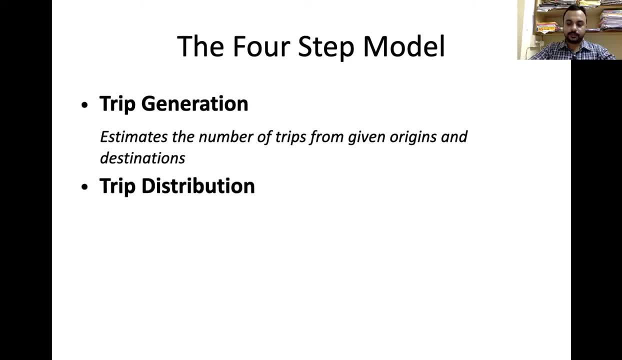 are going. that is trip instruction, butvis week distribution distribution. what the strip distribution does? it determines the destination for each trip: a to b or a to d, how many trips are going from this point to that point, of this point to that point. that particular study is that trip distribution. very simple, we'll move. 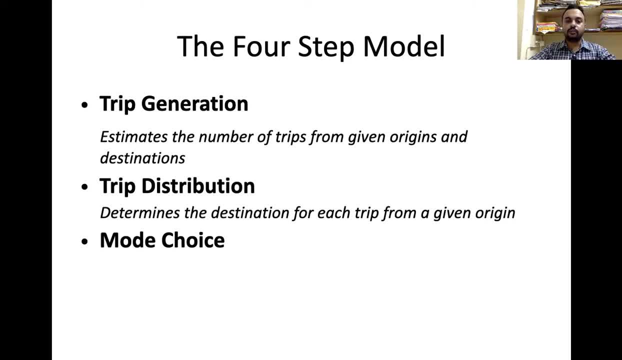 to the next important step of the four-step model, that is, the mode choice. so what is mode choice? so you have some particular mode of transportation. okay, basically, we are talking about road transportation. now we are not talking about road transportation. now we are talking about road transportation. no, we are not talking about 답 pyramid or work mode, when some particularようにассoscope we now sighs for the road TIM be, it depends on the size and type. 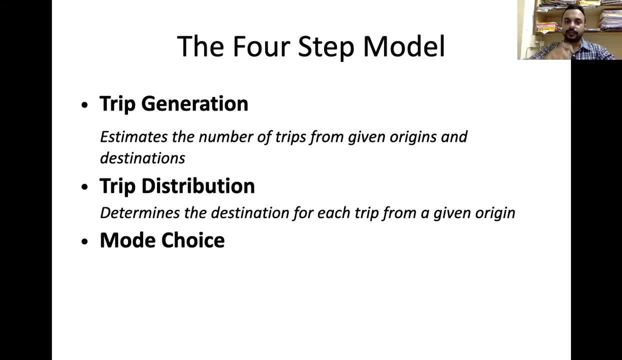 roadways, railways, airways and waterways. we're talking about the mode of transportation inside roadways only. what are the defined modes of transportation? so, basically, the mode of transportation is divided into two particular parameters. what are these? one is the public transportation. okay, that is city, bus, metro, rail, whatever. 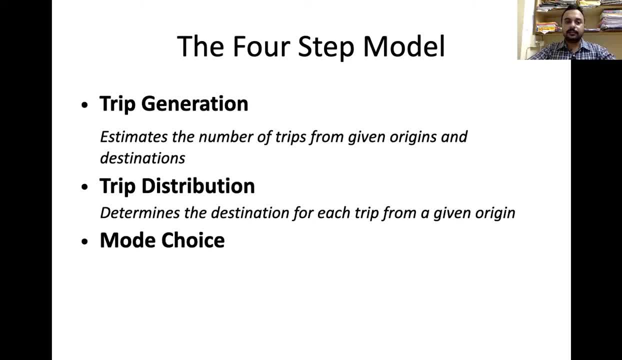 public transportation. you use auto rickshaws also maybe may come in public transportations- and another one is the private mode of transportation. that is, you use your own four-wheeler or two-wheeler as your mode. okay, so this mode choice determines the. 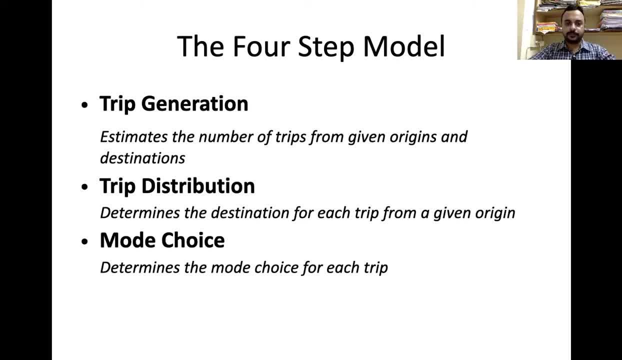 mode of transportation that you have chosen for your trip. okay, every person wants to travel at a the cheapest possible cost, so if the public transportation is adequate in your place, you might be willing to move in the public transportation. but sometimes, in many places, the public transportation is not adequate. 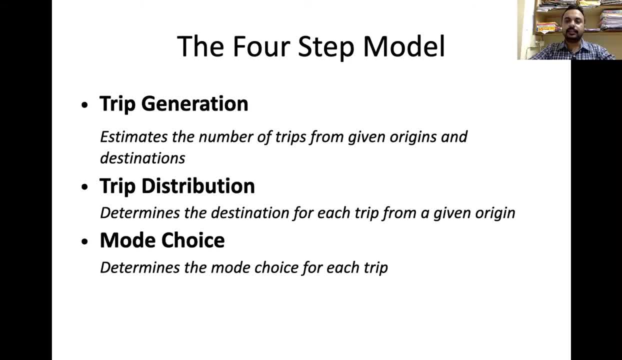 that the transportation that you can complete in 10 minutes by your own car or bike. it takes around 45 minutes by city bus. so you may prefer to use your own two-wheeler or four-wheeler in that particular case. so many things affects this mode choice. 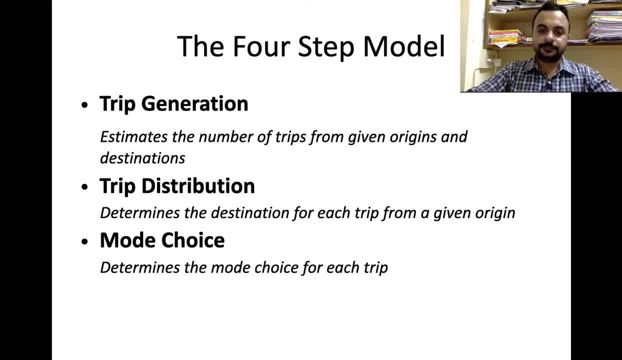 there are various models to study this mode choice also. okay, last step is the traffic assignment, or which also called as route assignment. that means, for example, we come while doing the trip distribution- you say that, suppose- from a to b. some like 10 strips are distributed from a to. 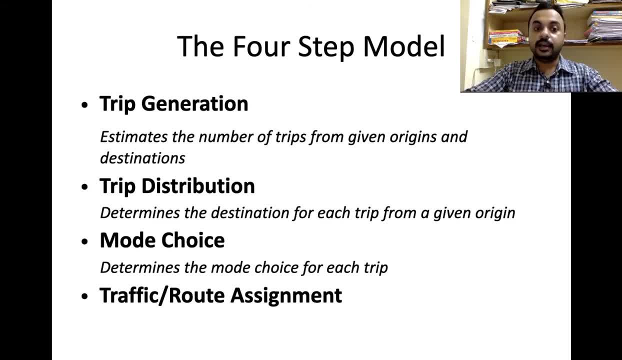 c, some five steps. the trips are distributed. but if, like suppose, 10 trips are going from a to b, how many routes are there to go from one place a to another place b? there may be some tree roads, okay, some different roads going through different stoppages. so which, which roads will you take? 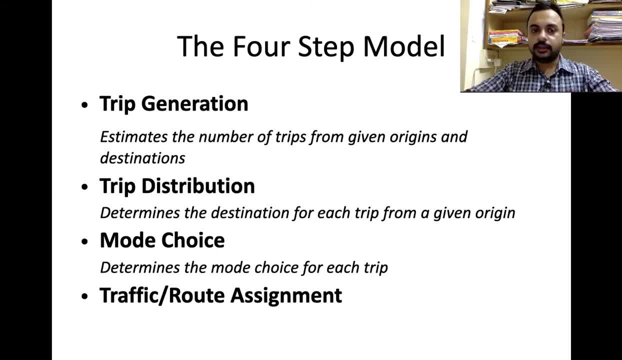 you will say i will take the shortest possible route. yes, people prefer to take the shortest possible route and another important factor people prefer is the comfort. if the shortest possible route is comfortable enough, you will prefer the shortest possible route. we prefer the routes having less amount of traffic. 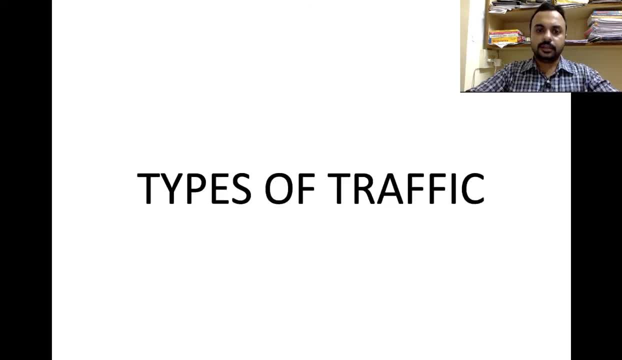 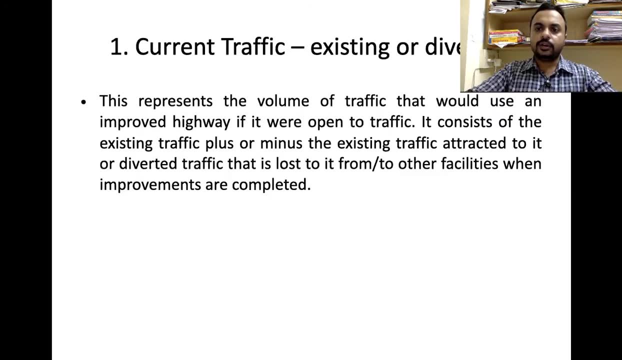 jams. okay, so next we are going to discuss about the different types of traffic. so one type of traffic is the current traffic, which is the existing or the diverted current traffic. this represents the volume of traffic that would use an improved highway if it were open to traffic. 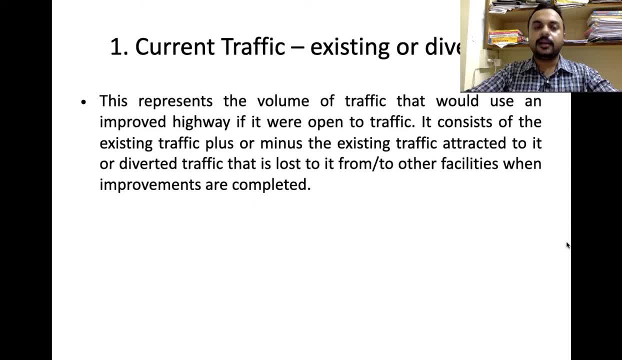 it consists of the existing traffic, plus or minus the traffic attracted to it, or diverted traffic that is lost from it to other facilities when improvements are completed- see current traffic means- which happens just after the construction, not predicted, but after the construction. if suppose one over bridge was being constructed from last two years. 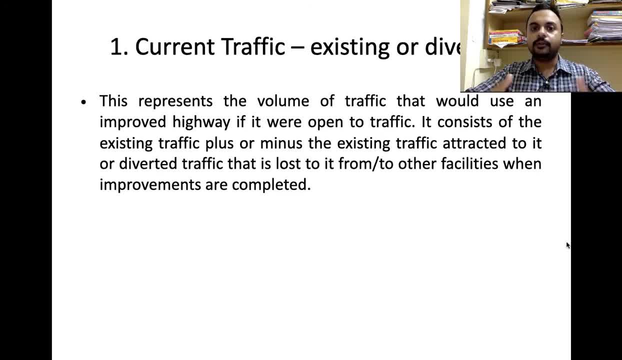 it is complete. the construction is complete. now we are focusing on the current traffic. so, see, you may see think that why will the- uh, what to say? traffic be diverted? there are various reasons that traffic may be diverted, because of some improved constructions also, okay, it might happen that there was another route which you were not following. 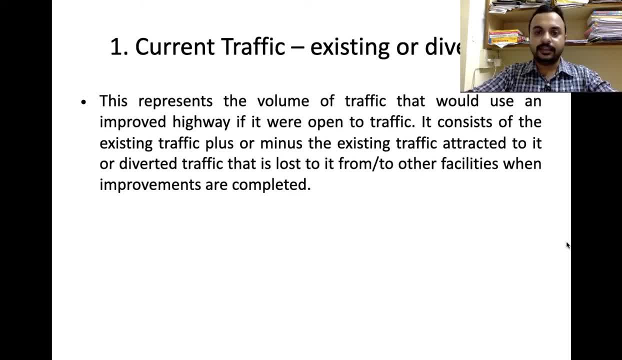 but now, when there is an improved route happening, the route which you are taking is now congested or there is a huge number of traffic and the people who were using route number two, now they are finding the route number one more short or more better for them. so now you might think that for me. 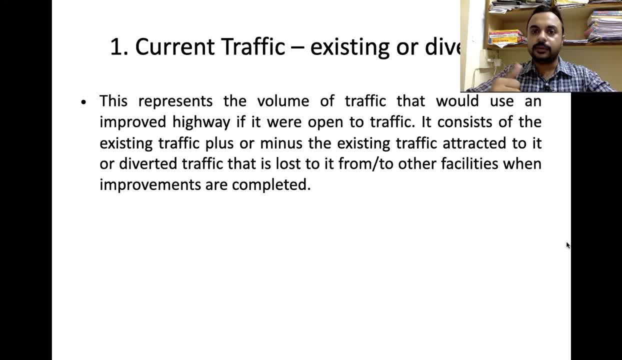 since my i was taking a longer route earlier than earlier. now route number two is now having less congestion, so better not to take a longer route. so route number two is shorter for me to reach from my destination. likewise, you are now diverted to another route, though there is an improvement because 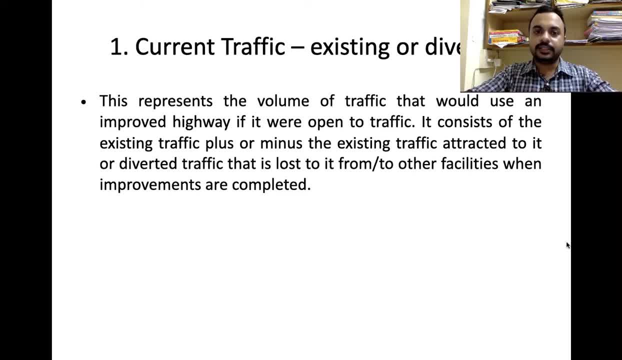 other people have come to this route and the other route, which has become less congested now. the other reasons may be like, for example, earlier you were moving this in this route free of cost and now there is an improved construction and you have to pay a toll amount of suppose. 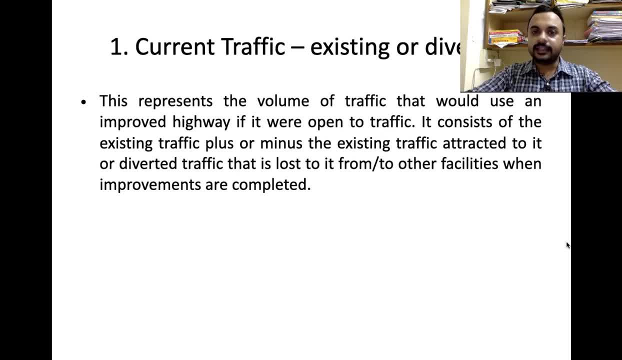 60 rupees. so you will think that better to take another route which is less comfortable. but i will save this 60 rupees of mine. 60, 60, 120 rupees i am saving in going and coming. so there are various reasons why the 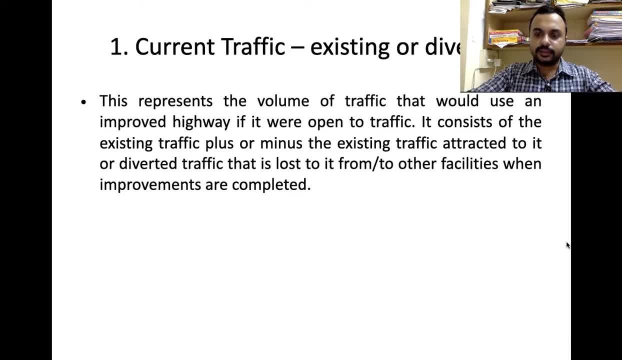 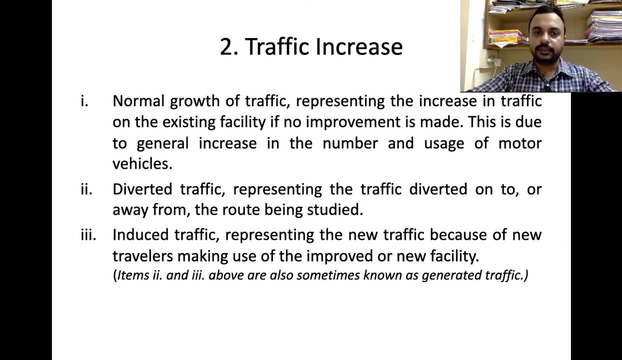 traffic also get diverted. so next type of traffic is the increase in traffic, that is, in the future, that what will be the increase or decrease in the traffic. okay, this is broadly divided into four subcategories. one is the normal growth of traffic, representing the increase in traffic on the existing facility if no improvement is made, if suppose you do. 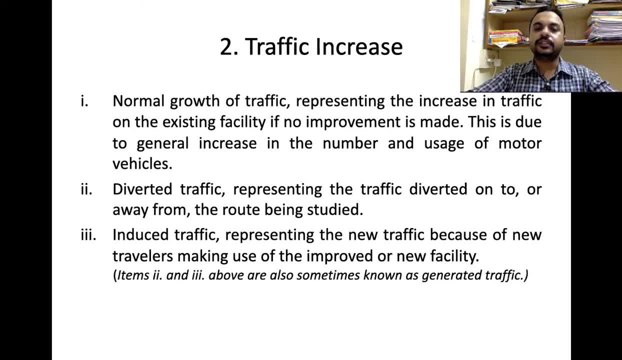 not construct the flyover, or if, suppose, you do not increase the width of the road or you are not constructing any facility, then also there will be an increase in the traffic. okay, this increase in the traffic because of increase in the urbanization, because of increase in the car ownership? okay, there are, there are. 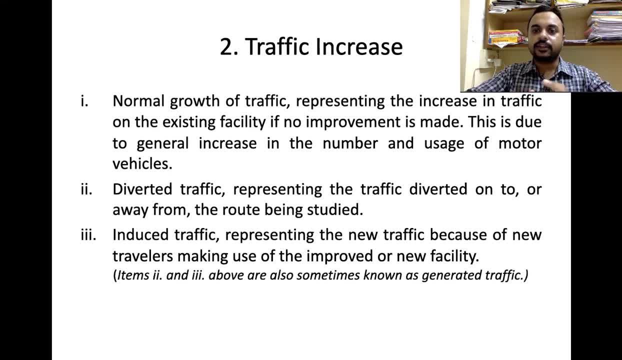 huge number of families which are buying cars for the first time every day. so, due to all this, there will be an increase in the traffic in spite, despite, of any kind of facilities being construct, constructed. the next type is the diverted traffic, representing the traffic diverted onto or away from the route being studied. so, as i have already said, that there may be. 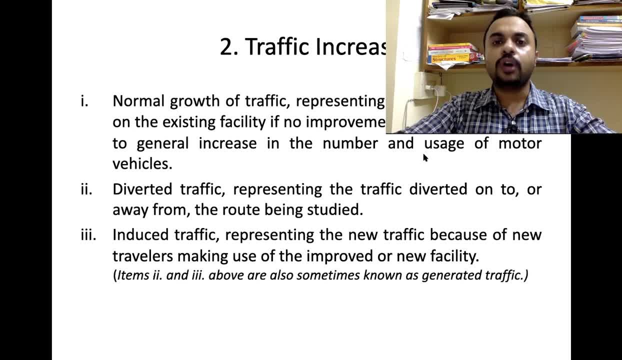 some diversion of the traffic. so how much traffic is being diverted? that type amount is called the diverted traffic. next is the induced traffic, representing the new traffic because of new travelers making use of the improved or new facilities. obviously, because there is a new facility, it's a better route, it's a better construction, so obviously there will be. 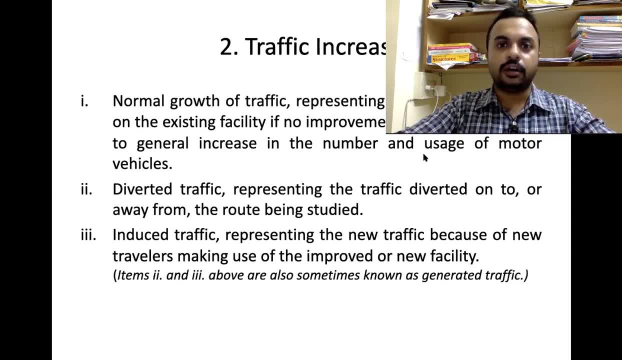 new traffic because of the construction of the road. maybe new offices have come up in those areas again to join that office. there will be new employees, so they will be taking the road. there will be different people who were earlier taking different roads, but not they will choose to take this road because of its improved 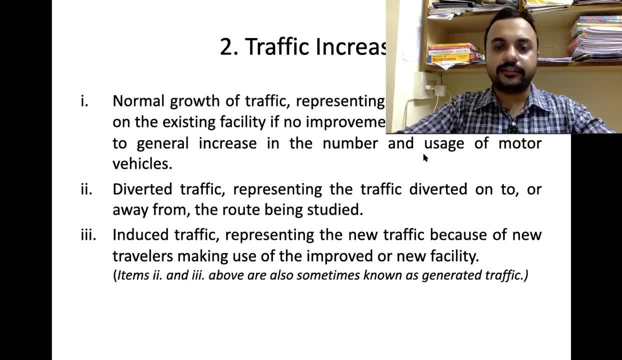 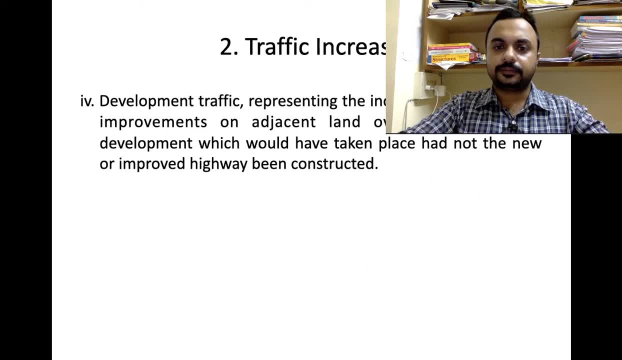 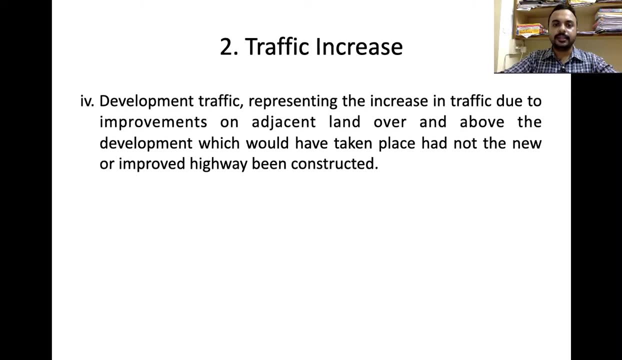 condition. so this induced and diverted traffic is known as the generated traffic. okay so, so now next is the development traffic. okay so, development traffic. it represents the increase in traffic due to improvements on adjacent land, over and above the development which would have taken place had not the new or improved highway been constructed. 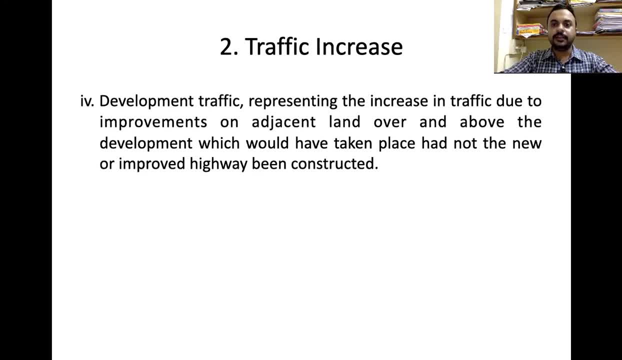 in the past. obviously there will be a traffic which will be occurring in this particular route because of the development in some other areas. okay, there, if some other construction, other roads are constructed, other, better roads are constructed in another area adjacent to this road, obviously the people to go to that better road maybe take will be taking this. 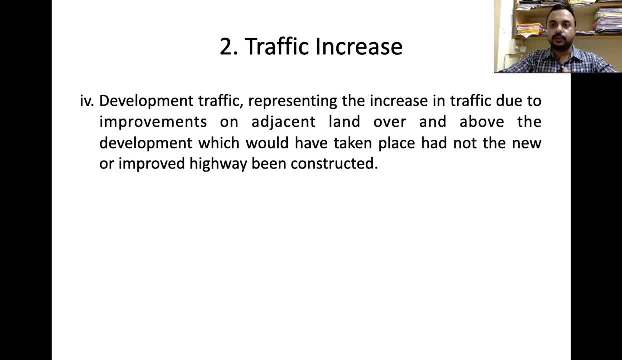 particular road. okay, that effect on this particular road, suppose i am telling this is road number one and another one is road number two. so there is a number of people who will use road number one to land into road number two and go to some other places. so there is an improvement in road number. 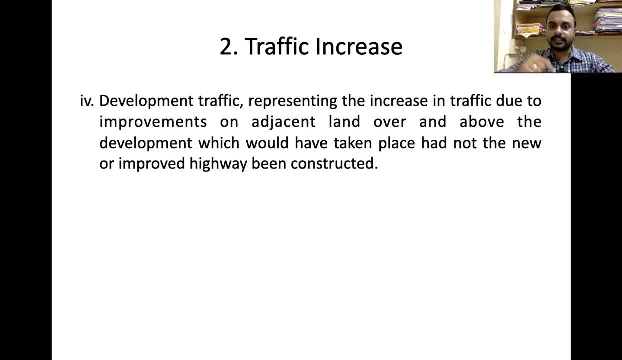 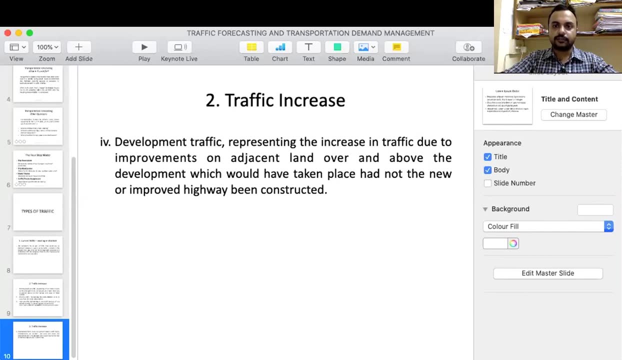 two, but simultaneously there is an increase in road number one. so this kind of traffic being generated is known as development traffic. so i hope the concept is clear. so with this we have come to the end of the discussion of transportation forecasting and traffic forecasting and transportation demand management. we have seen very clearly that traffic is 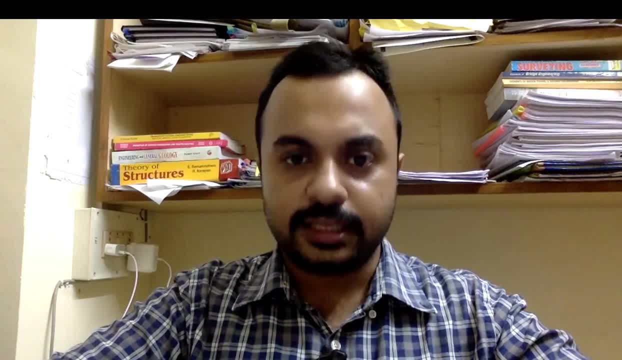 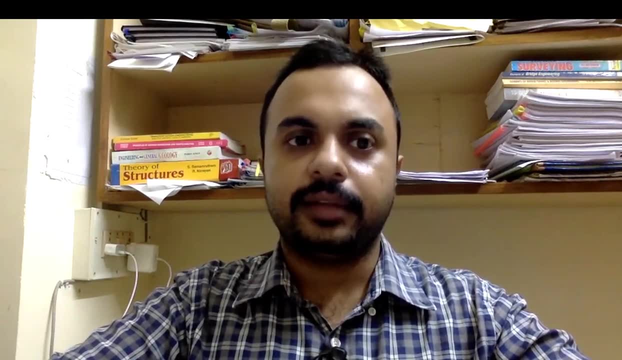 management. we have seen very clearly what are the four-step processes and why forecasting is important and why what are the different types of traffic. so with this we would like to conclude for today, thank you. thank you so much.